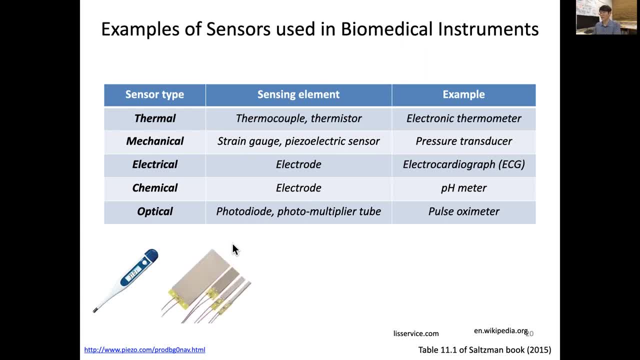 can give rise to a voltage. So here's an example, as I put this piezoelectric transducer which when we apply a voltage then this piezo will have a change. so in this case are changing in displacement. So an example as a pressure transducer, one type of pressure transducer. I. 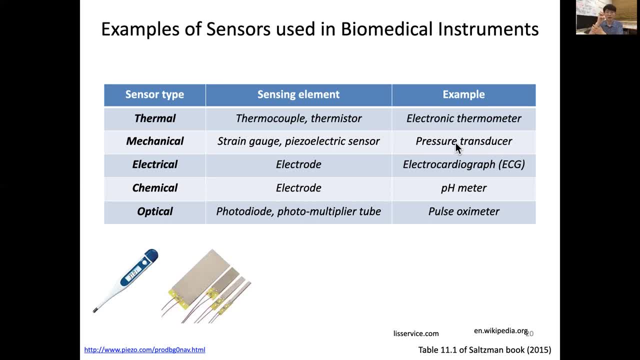 actually use is a piezoelectric So that we measure, let's say, gas pressure. in a specific vessel. There's a specific gas and I want to measure the gas, to measure the pressure. we have a piezoelectric transducer that measures this pressure gives rise. 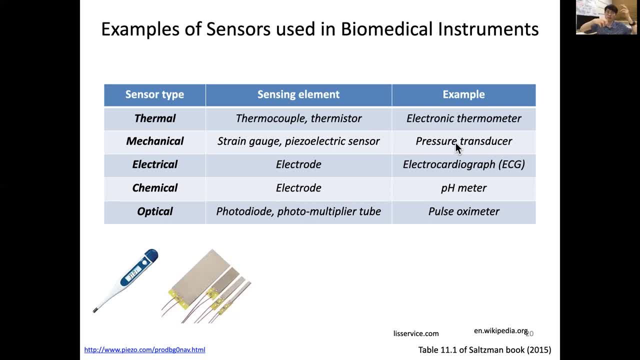 to a voltage difference and that we can measure. so that's another example of pressure transducer. you see, transduce means converting one type of signal into another form. and thirdly, electrical sensor, uh. one example is electrode uh, for example, like electrocardiography and and that's like this you you have. we have already discussed these electrodes are sensing. 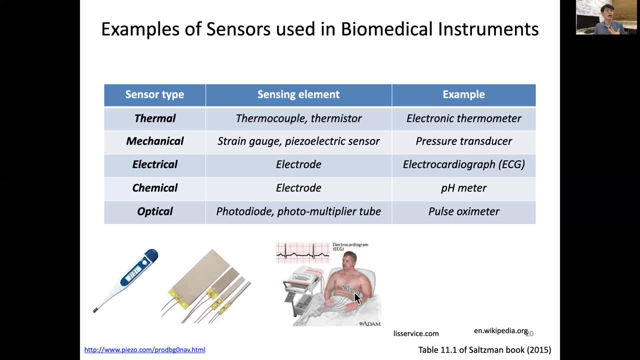 the electrical activity of our heart, because the heart cardiac myocytes generate electrical field and electric vectors and chemical sensor or an example. as a sensing element. we can also use our electrode especially and put example is a ph meter which looks like this: uh, many laboratories have this. when you are preparing a solution with a certain ph, 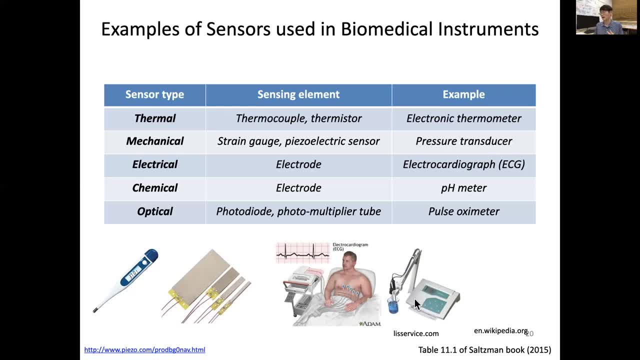 then you have to use this ph meter to measure the ph, and these are the electrode. and lastly, i want to discuss about optical sensor and sensing element which measures the, the photon, the amount of photons or light. so uh one, a typical one, is so called a photodiode, which is uh cheap and 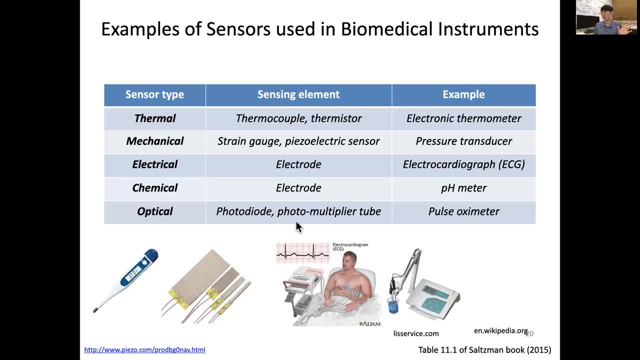 broadly used, and the other, more specialty ones, are photo multiplier tube, which is a very, very sensitive, even giving us a single photon sensitivity. so we'll discuss more about this. and what are the example of this optical sensor? and one of the vital sign and important one is the pulse oximeter. now, the pulse oximeter uses a light to uh having this transmitting. 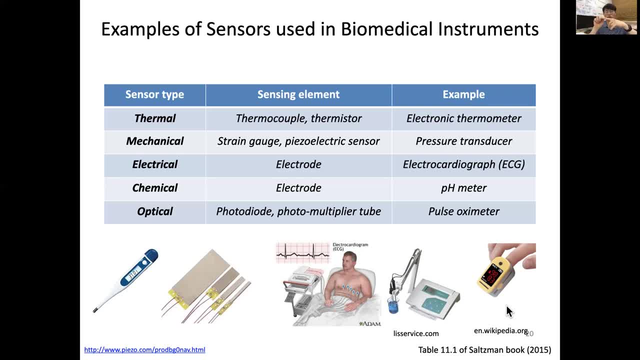 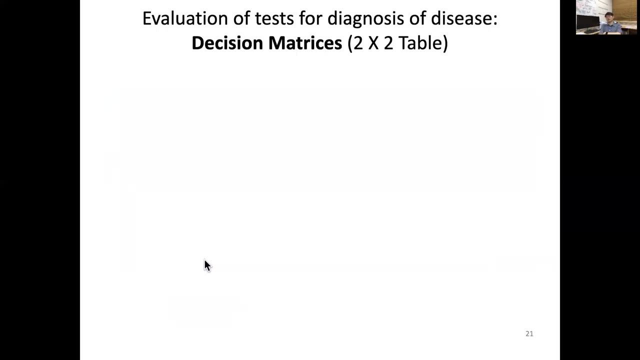 through our, uh, let's say, biological tissue, where there exists a blood vessel, so that we can measure the oxygen, uh, concentration, saturation of the oxygen in the tissue. okay, so now let's discuss about when we develop a new diagnostic test. let's say we have this machine which, let's say, measures, uh, some body fluid or 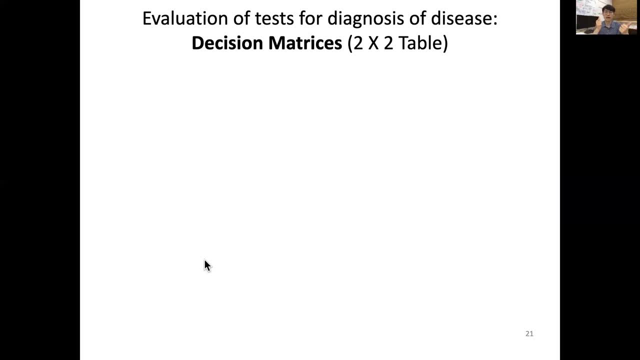 patient and it gives out a result saying that, hey, you've got this disease or you are free from the disease. then how can we uh, um, how can it characterize the performance of this diagnostic test? so for this, uh, people have developed a very simple decision matrix. so this is a matrix, is about like this. so first, uh, in an absolute sense like the patient, 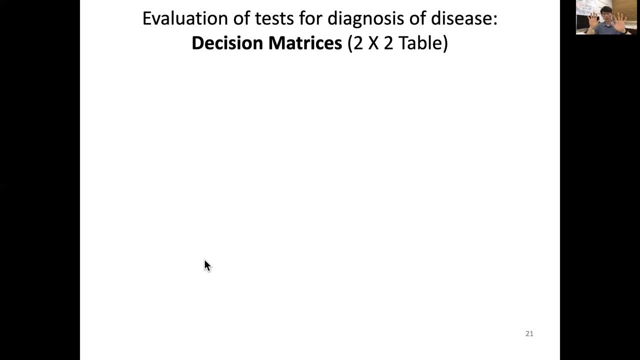 will have this disease or no disease. so that's what we ultimately want to know. however, that's not very easy to figure out. so we develop an instrument or bio instrument which speaks out the result as a value, quantitative value that we will, based on these very rules. 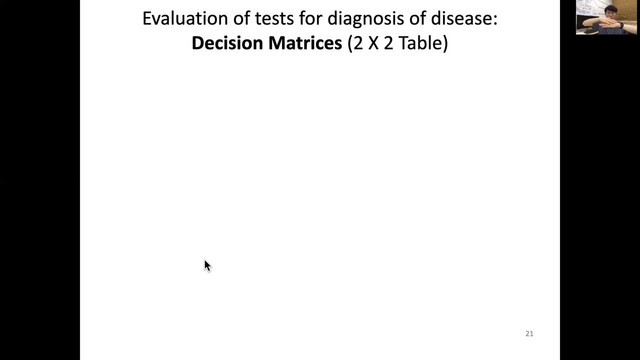 so we can say, hey, this is a threshold and you are higher than this value, hey, you are positive, which is like we from our test or below, that's a negative. so positive and negative of our disease, uh test results and the absolute sense of disease, present or absent, and with those two by two table. 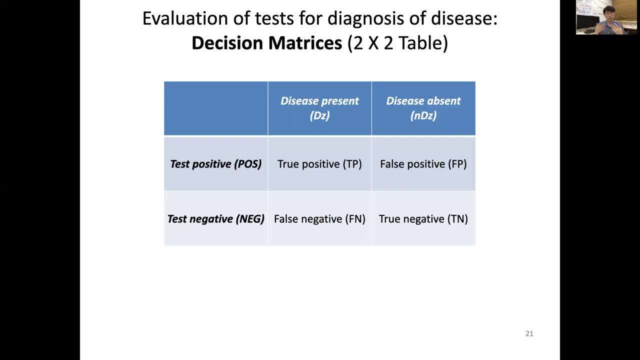 we can now characterize our uh performance of uh, this instrument. so here you see, this is present or this is absent, and disease and no disease, while test side we can always set certain criterions and having it as a test positive or test narrative, that with this what we can say, what we are interested in, what the true disease. 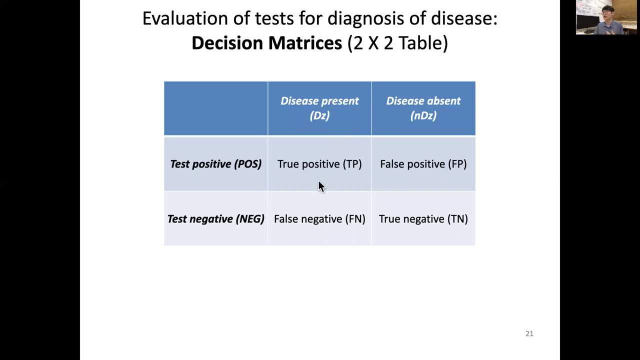 or not. so having disease and getting positive means true, positive makes sense, having no disease and getting negative is true, negative. so these are like the true, true estimation. and while there are other cases having i don't have a disease but somehow this test results giving me damn positive. so that's false, positive. okay, but i do have a disease. but this machine is. 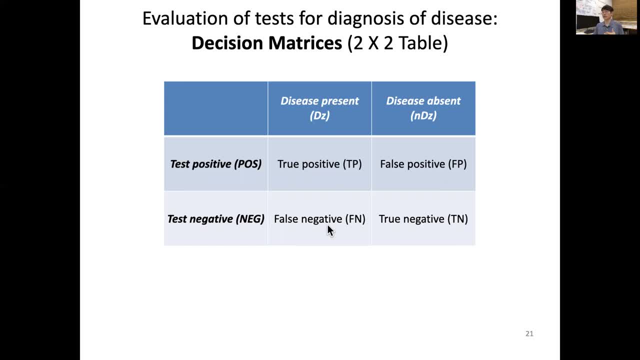 not good enough to giving me a negative. that means a force negative. does that make sense? so this is very simple. um, this is a matrix which gives us to define more specific performance matrix. so for this, like we can say, like all or everything, every case is disease plus no disease. 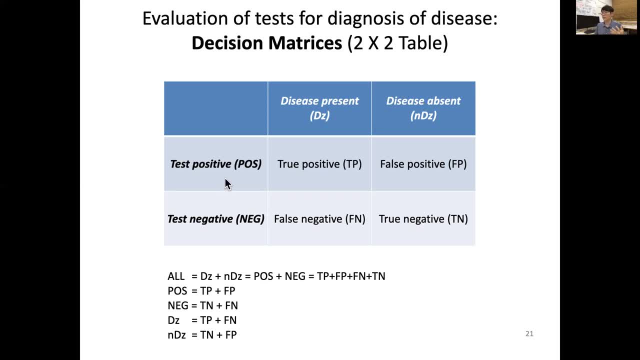 right, or we can say there's only positive or negative. so all the positive plus negative, which means all these four elements. so true positive, false positive, false negative, true negative. So that's all. And what are the positive? So positive is true positive plus false positive. Okay. 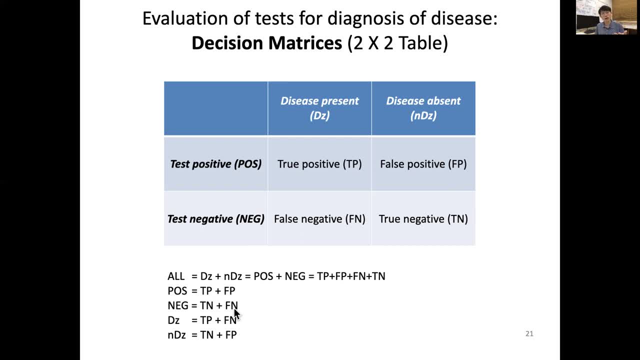 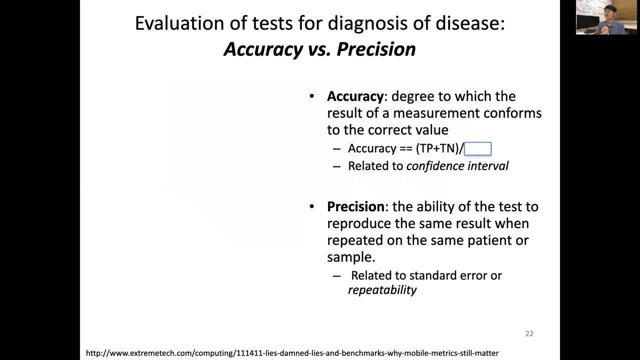 What are negative, True negative plus false negative? What are the disease? So disease can compose of true, positive plus false negative. Likewise, no disease will be composed of false positive plus true negative. So with this we will define more specific parameters. So for that let's consider about: hey, what's the 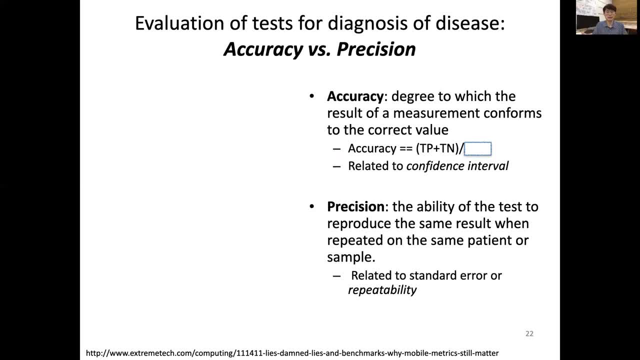 accuracy of your test or your machine. Okay, So for diagnosis of disease, the accuracy can be defined as the degree to which the result of a measurement confirms the correct value. How accurate? How can this machine give the correct value? So we are more interested in correct value, which means 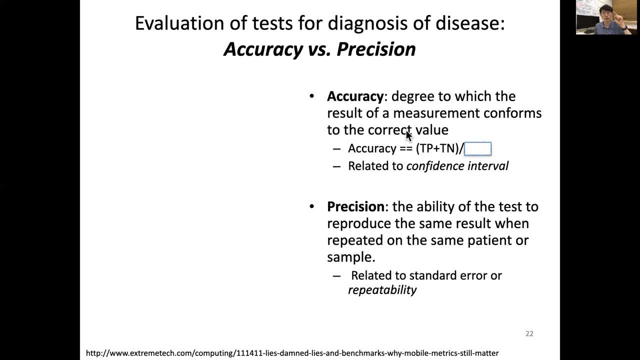 in the disease matrix, the correct one is always true, So that accuracy can be defined as true, positive plus true negative. case Out of what? All the cases? So that's all. So why it's all? Let's see Disease, no disease, positive, negative. We. 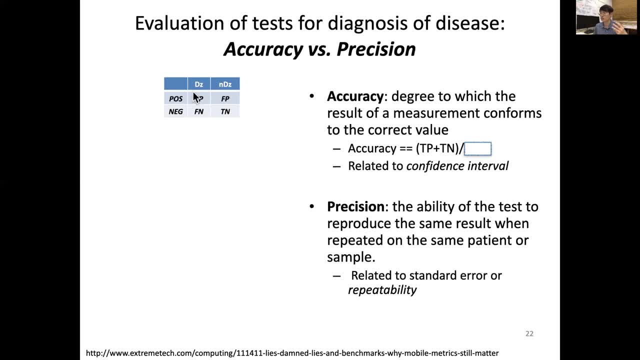 are interested in the proportion of true, positive and true negative. So we are interested in the proportion of true, negative out of all. Okay, So that's all means everything. And this also relates to confidence interval, which means to the what interval the true value of this population will lie, likely to lie So, and the other? 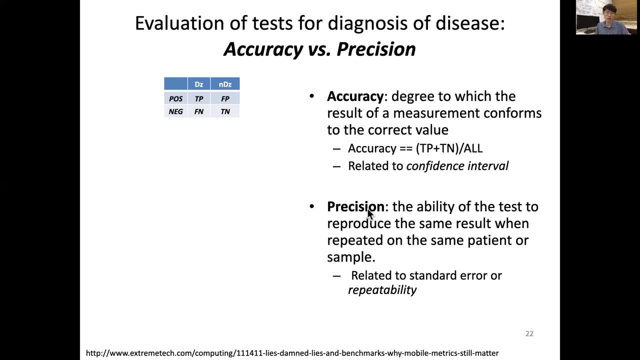 aspect we've already discussed- and I'm talking about precision- is the ability of test to reproduce the same result. So let's say I want to measure my height, So I'm having a ruler to measure my height once and I write down the result And I do measure it again Second time. oh the. 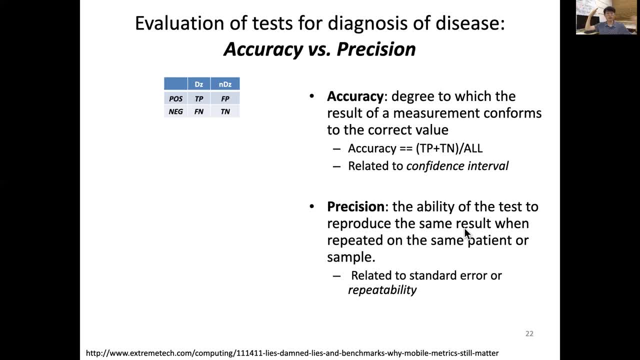 value will not be always the same. Let's say, another person came in to measure it and that values are also different. So you know, this is the like: any instrument we, we are measuring, you will not have exactly the same value. So there comes the concept of 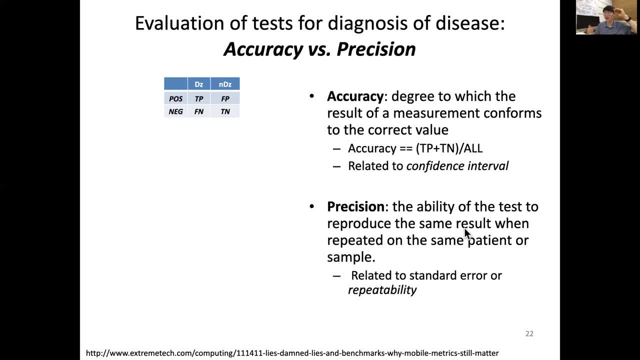 how repeatable those measurement values are that we call as a precision when repeated on the same patient or sample. So that's related to really standard error or standard deviation or repeatability issue of our instrument. So that's a simple diagram which I call it. 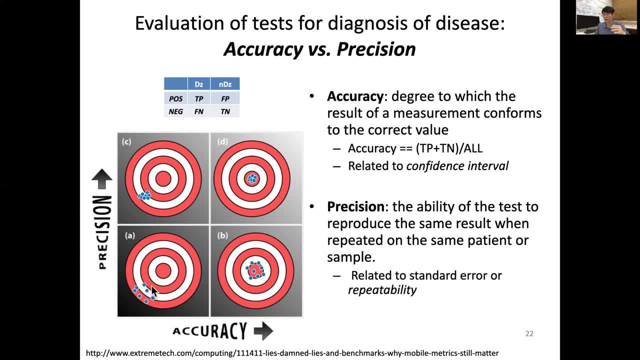 again. You see, the distribution of the results will be more compact. Distribution is more compact. So, upon this, C and D is higher precision, While we also accuracy matters. the mean is not at the center, So this mean is not the center. So this is even high precision low. 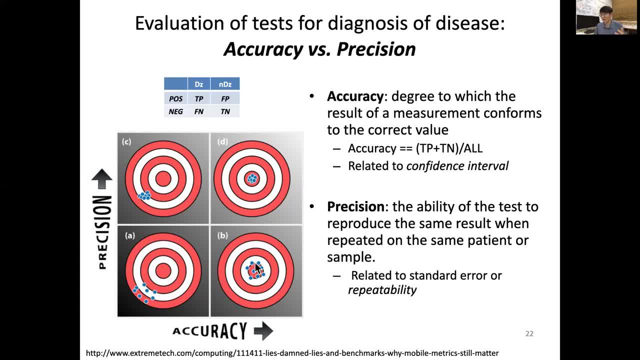 accuracy. However, this is great And in this case, hey, it may not be precise, but when, when you measure it over and over, There's a great possibility. with this you can make a mean value to represent the center. 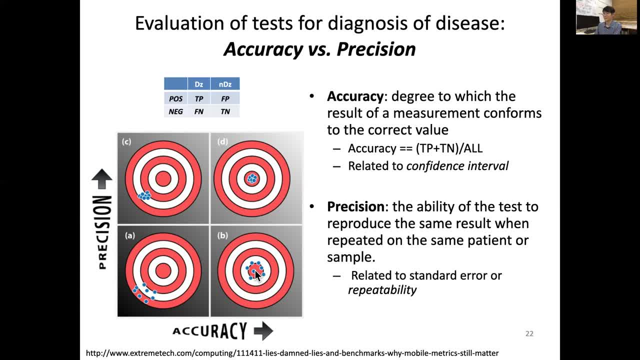 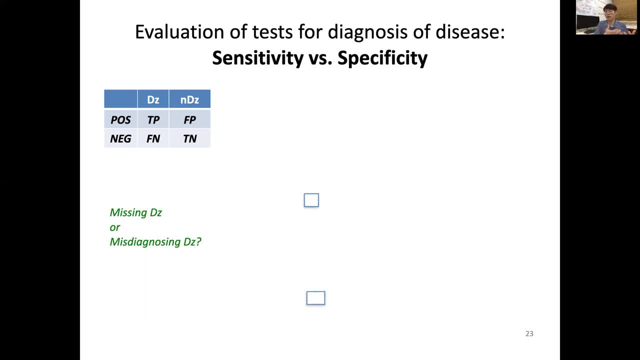 That will be pretty accurate. Okay, So now I want to discuss: when you are developing a bioweapon instrument, which is for, let's say, disease diagnostics, you want to get a prover. then the people who want to buy or commercialize your device will ask you: Hey, what's the sensitivity and specificity? 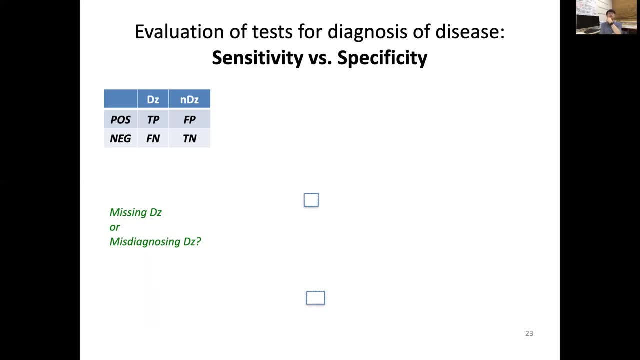 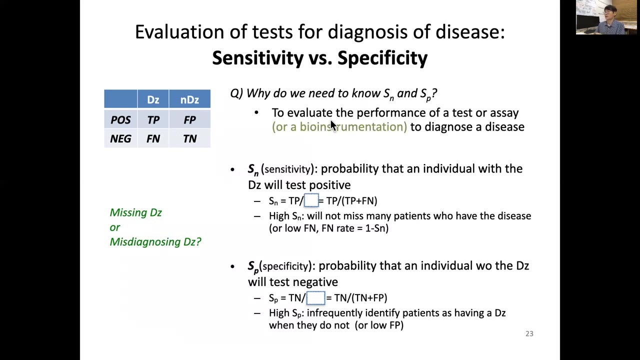 of your device? Yeah, instrument. then wait a second. what? what is sensitivity and specificity? okay, so we have to know the definition first. so there's a simple two by two. this is a matrix, and let's see why we need to know about sensitivity and specificity. so that's what people will ask you. so to evaluate the 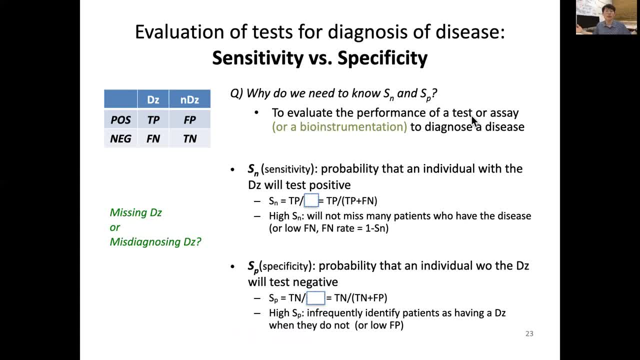 performance of a test or essay, or by instrumentation, what you have to diagnose a disease. these are the important parameter, which belongs purely to that instrument. okay, so the definition of sensitivity is the probability that an individual who has a disease we want, who have the disease to test positive. that's sensitivity, okay, so 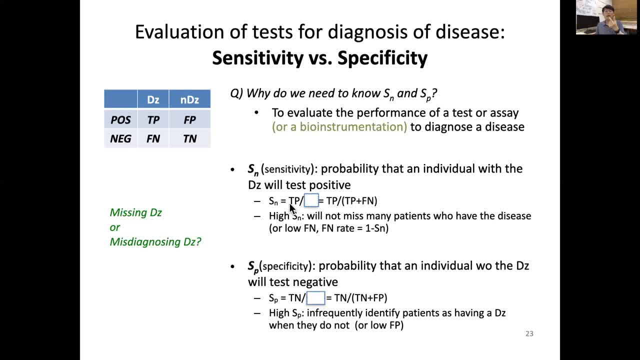 how do we define sensitivity? yeah, the amount of true positive among those who have a disease. so sensitivity only matters for a population who have the disease. so that disease and this is composed of true positive plus force negative. from this formula you can see: higher sensitivity means you have low force negative and force negative means those. 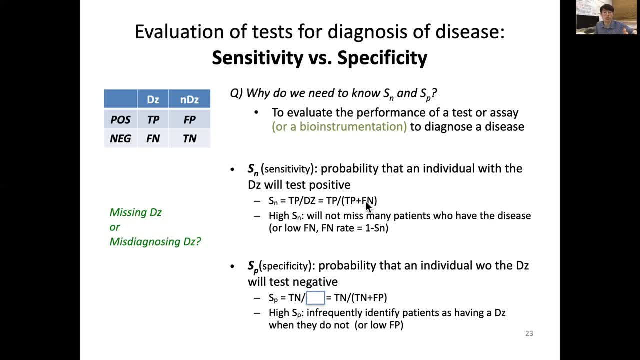 who have a disease but test turns result turn out to be negative. okay, that's force negative. so what does high sensitivity mean? that means if you truly have a disease, this device is likely to give you positive result. okay, so that we, this high sensitivity device, will not. 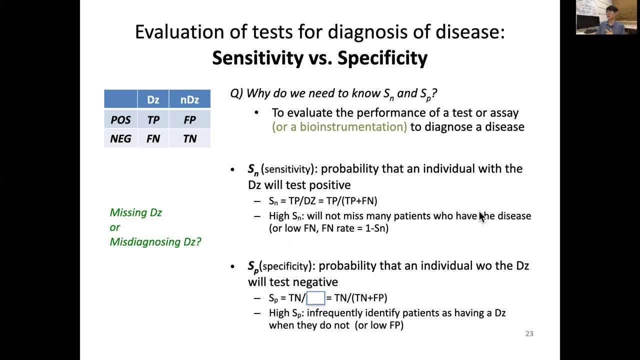 miss many patients who actually have the disease. okay, or which means low force negative or force negative rate. if you take one minus sn, then will be force negative out of those disease. so sensitivity really means we are curious about: hey, someone has disease and this test should give you a positive results. that's about sensitivity. then you can think of the opposite case. 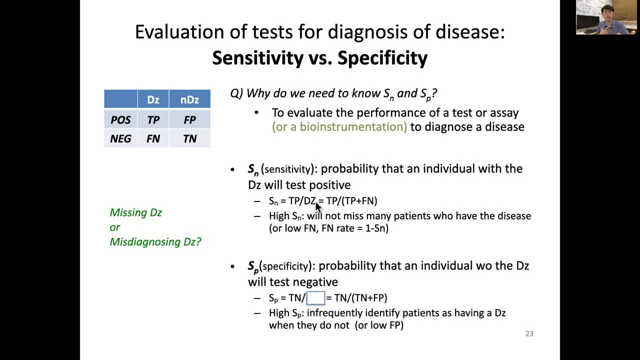 hey, i don't have a disease and i have this test and i want to have a negative results. okay, so that is related to specificity. what it defines is probability that an individual who do not have a disease will test negative. so that, hey, the definition of specificity should be: hey, someone who has no disease will test negative, so no disease out. 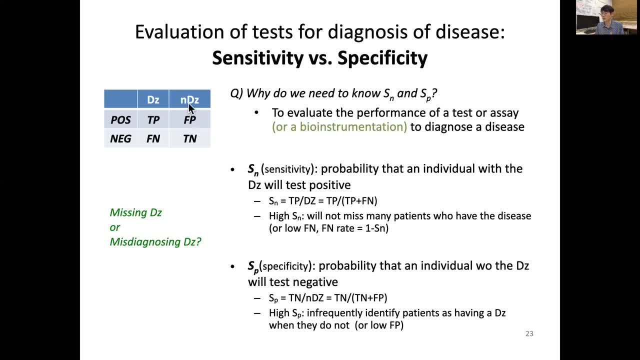 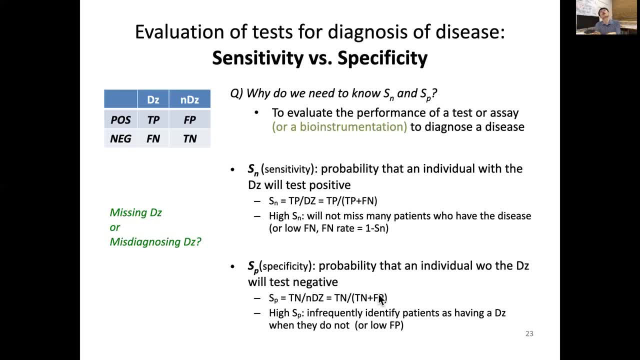 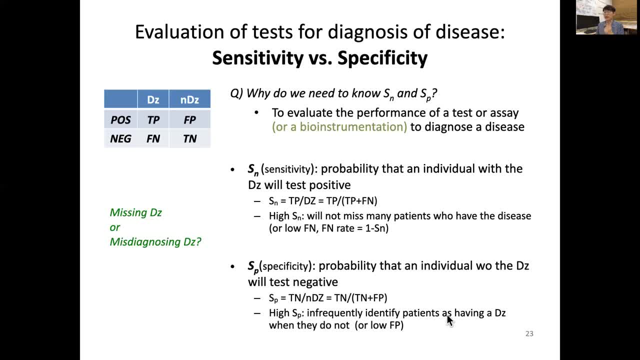 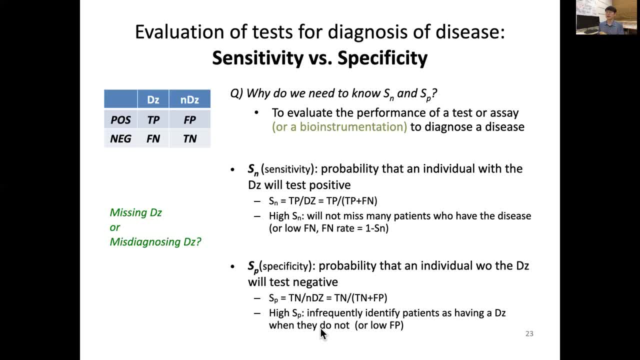 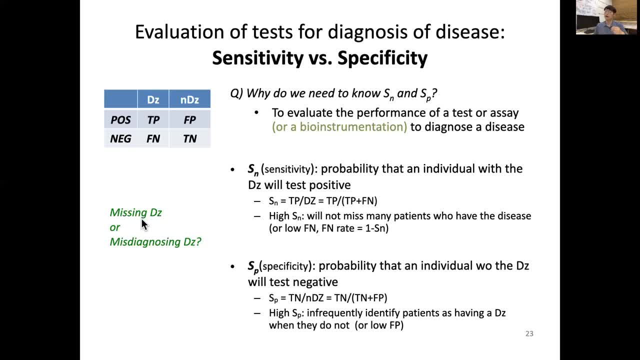 okay, so this is the definition of high sensitivity. okay, so this is the definition of high sensitivity: you are less likely to miss the disease. you are less likely to miss the disease. you are less likely to miss the disease by using this instrumentation, by using this instrumentation, by using this instrumentation, on the other hand, high specificity. 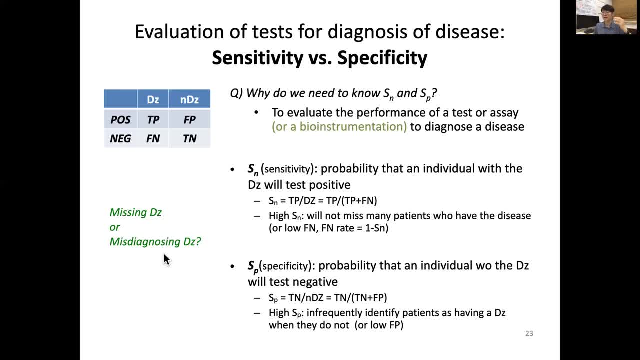 on the other hand, high specificity. on the other hand, high specificity means you are. this test will less likely to means you are. this test will less likely to means you are. this test will less likely to miss diagnose a disease, so it's quite. miss diagnose a disease, so it's quite. 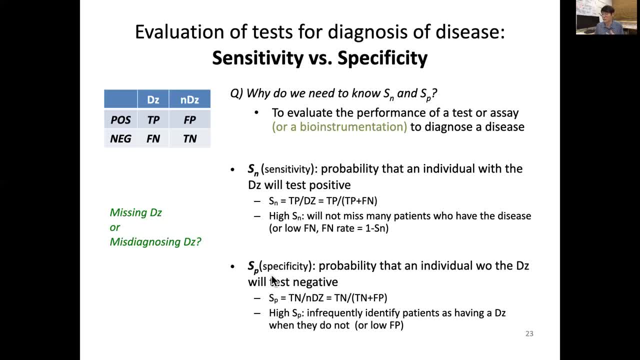 miss diagnose a disease. so it's quite important, but it can be also confusing. important, but it can be also confusing. important, but it can be also confusing. so specificity involves only those. so specificity involves only those. so specificity involves only those population who do not have the disease. 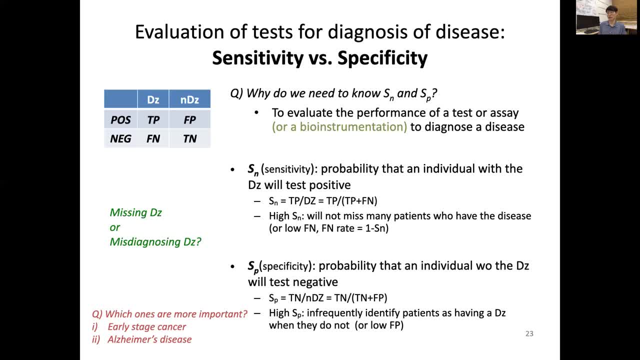 population who do not have the disease, population who do not have the disease. okay, so let me give you a quiz a quick. okay, so let me give you a quiz a quick. okay, so let me give you a quiz, a quick quiz, quiz, quiz. so in, i will talk about this. 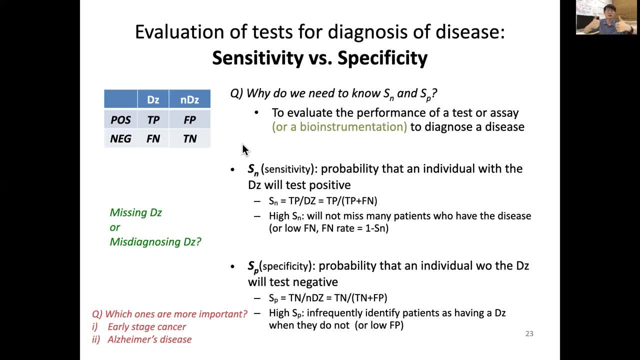 so in, i will talk about this. so in, i will talk about this. you know both sensitivity and specificity. you know both sensitivity and specificity. you know both sensitivity and specificity. higher the better, but unfortunately, higher the better, but unfortunately, higher the better, but unfortunately there is always a compromise which i 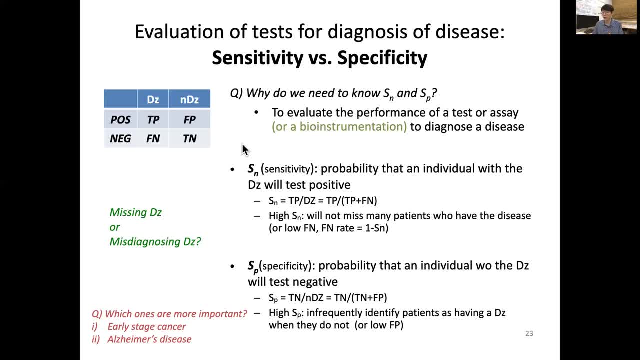 there is always a compromise which i there is always a compromise which i will discuss, will discuss, will discuss next time, but let me ask your question next time. but let me ask your question next time. but let me ask your question: which ones are more important? which ones are more important? 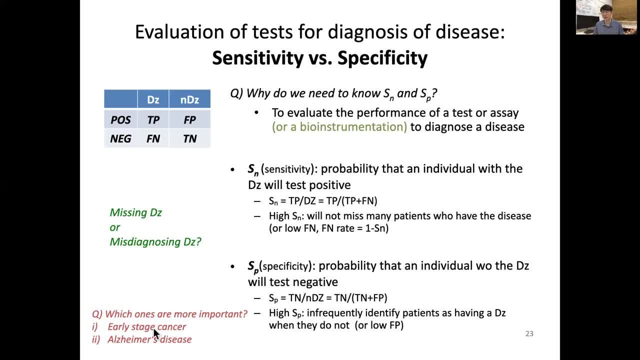 which ones are more important, between sensitivity or specificity? let's between sensitivity or specificity. let's between sensitivity or specificity. let's say say: say early stage cancer and think about the early stage cancer, and think about the early stage cancer and think about the disease of early stage cancer. 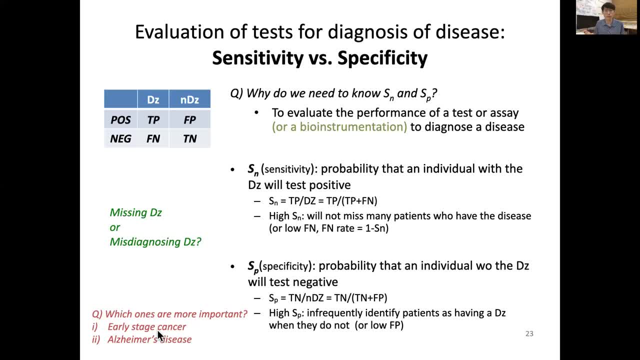 disease of early stage cancer. disease of early stage cancer means cancer is very, very important. means cancer is very, very important, means cancer is very, very important disease because it can be fatal disease, because it can be fatal disease, because it can be fatal so early stage, if you don't diagnose. 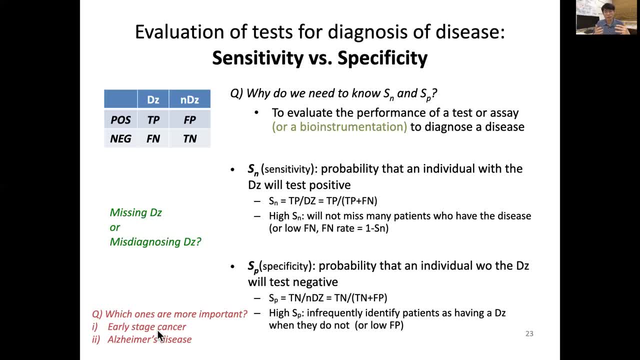 well enough. for example, if you miss the well enough. for example, if you miss the well enough, for example, if you miss the early stage cancer, early stage cancer, early stage cancer, then it turns out to be real cancer, then it turns out to be real cancer, then it turns out to be real cancer later on. 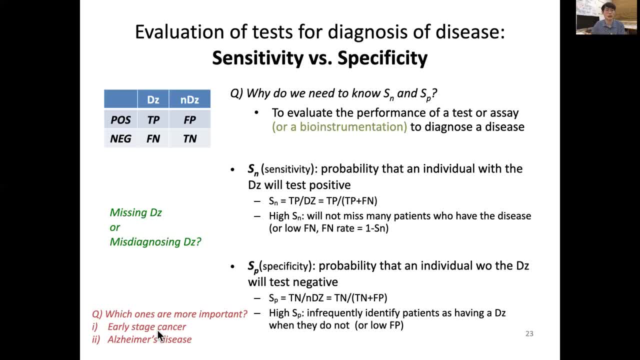 later on, later on and later stage- you already know it's. and later stage- you already know it's. and later stage: you already know it's more fatal, more fatal, more fatal. so it's very important you do not miss. so it's very important you do not miss. 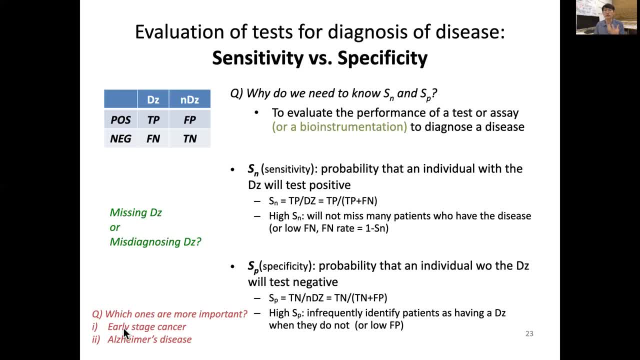 so it's very important you do not miss the disease because the disease, because the disease, because you can change. you can treat at the you can change, you can treat at the you can change, you can treat at the course of disease if you find it at an. 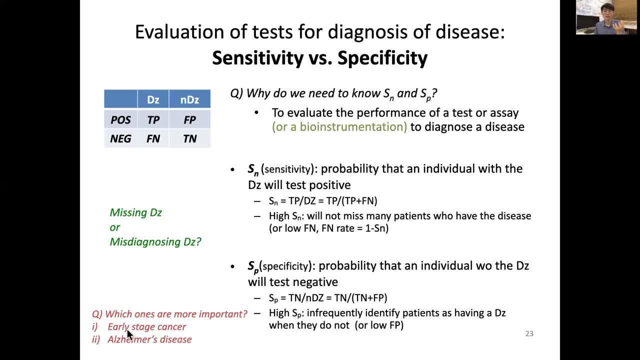 course of disease, if you find it at an course of disease, if you find it at an early stage. so if you have a test which early stage, so if you have a test which early stage, so if you have a test which will diagnose early stage cancer, will diagnose early stage cancer. 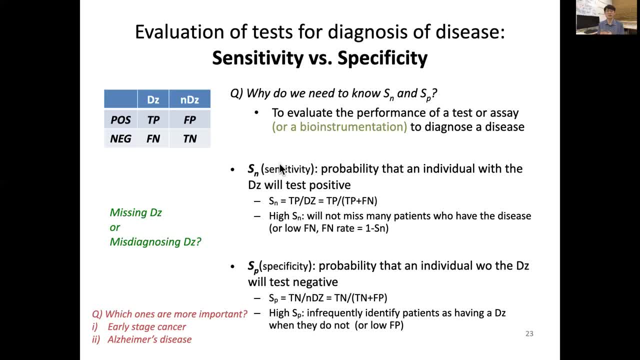 will diagnose early stage cancer. you make sure you have a high sensitivity. you make sure you have a high sensitivity. you make sure you have a high sensitivity. does it make sense? does it make sense? does it make sense? let's think about another type of disease. let's think about another type of disease. 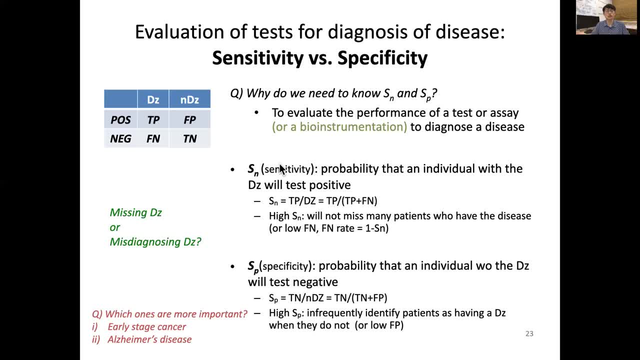 let's think about another type of disease. let's say there's no. let's say there's no. let's say there's no, uh, a good cure of the disease. no, uh, a good cure of the disease. no, uh, a good cure of the disease- no treatment. 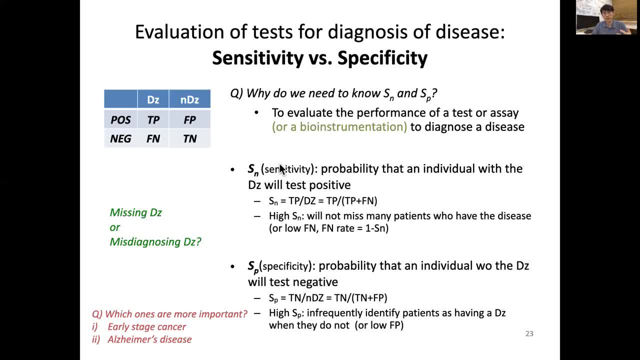 treatment, treatment, okay. so even if you know that you have okay. so even if you know that you have, okay. so even if you know that you have a disease, if there's nothing or not a disease, if there's nothing or not a disease, if there's nothing or not many things to do. 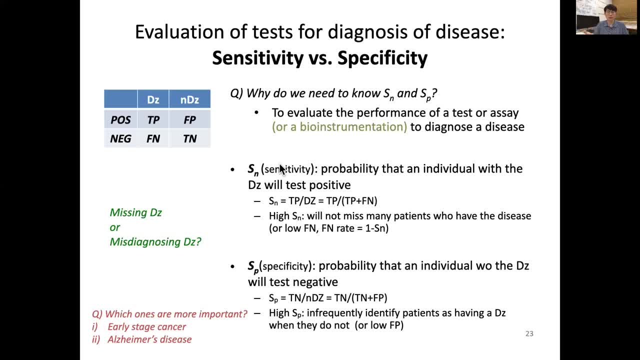 many things to do, many things to do for the patient that will aggravate for the patient. that will aggravate for the patient. that will aggravate the patient or give burden to the the patient, or give burden to the the patient or give burden to the patient. 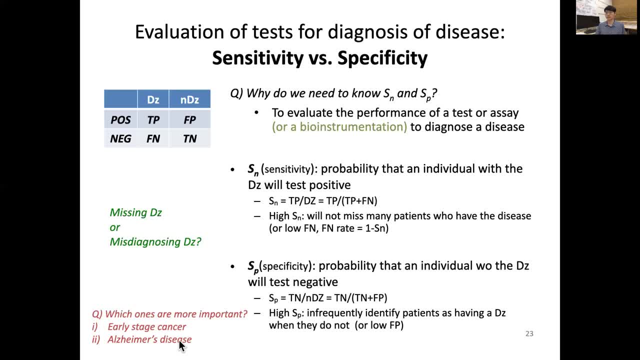 patient, patient, so. so here's an example. let's say so. so here's an example. let's say so. so here's an example. let's say: alzheimer's disease, alzheimer's disease, alzheimer's disease to date- uh, you know if i know that. to date, uh, you know, if i know that. 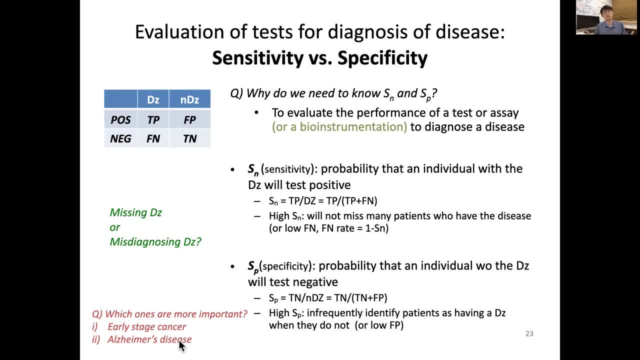 to date. uh, you know, if i know that, like i've got alzheimer's disease, like i've got alzheimer's disease, like i've got alzheimer's disease, there's not much thing i can do then there's not much thing i can do then. 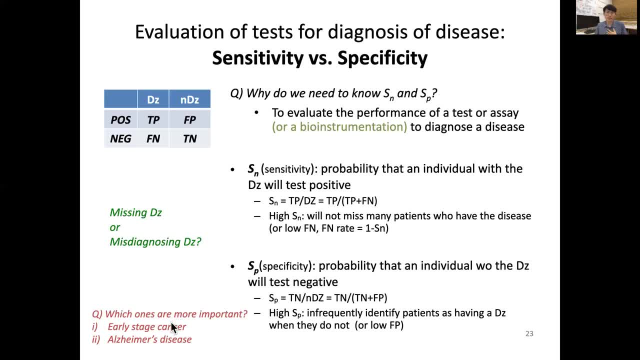 there's not much thing i can do. then what if? if i misdiagnose it, so i? what if? if i misdiagnose it, so i? what if, if i misdiagnose it, so i actually do not have alzheimer's disease, actually do not have alzheimer's disease? 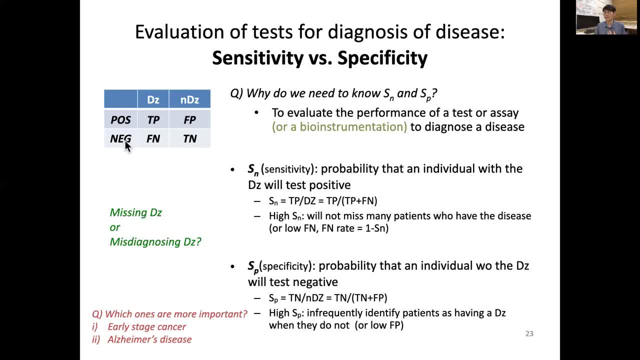 actually do not have alzheimer's disease, but this test will give me. but this test will give me, but this test will give me a positive, so which is a false positive, a positive, so which is a false positive, a positive, so which is a false positive, then, 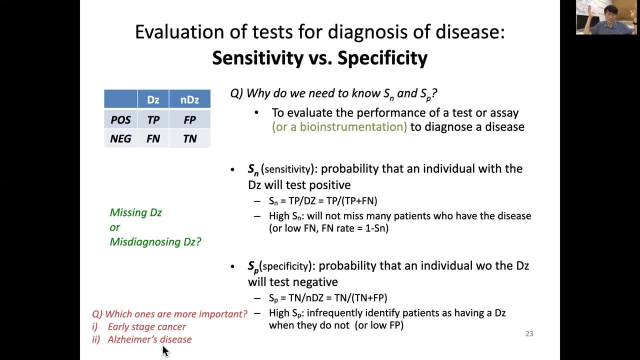 then, then, oh, because of this, i feel, oh, because of this, i feel, oh, because of this, i feel you know, i have to know whether i really you know, i have to know whether i really you know, i have to know whether i really have alzheimer's disease with this test. 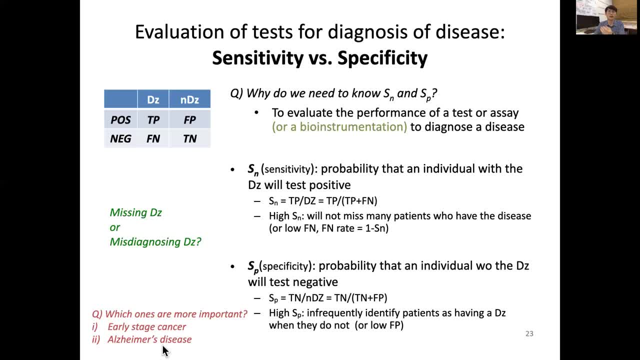 have alzheimer's disease with this test. have alzheimer's disease with this test, so i have to undergo. hey, i need a more, so i have to undergo. hey, i need a more, so i have to undergo. hey, i need a more more accurate test, which will be costly. 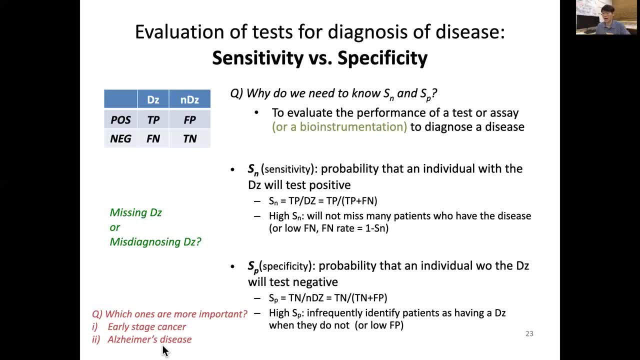 more accurate test, which will be costly. more accurate test, which will be costly. so i undergo follow-up exams. and so i undergo follow-up exams, and so i undergo follow-up exams. and that gives me more burden. that gives me more burden. that gives me more burden. okay so, but the problem is, even if i 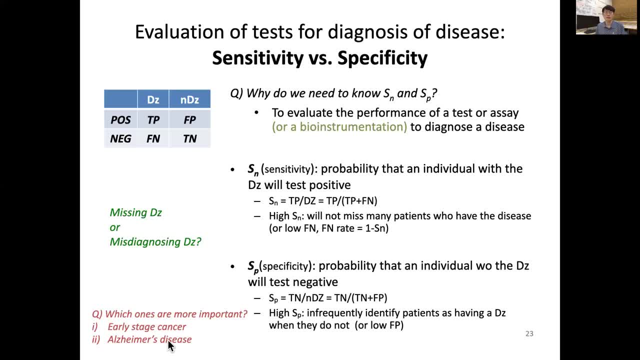 okay so, but the problem is, even if i- okay so, but the problem is, even if i got- uh, i'm truly getting the alzheimer's got. uh, i'm truly getting the alzheimer's got. uh, i'm truly getting the alzheimer's disease, disease, disease. there's not much thing to do so in this. 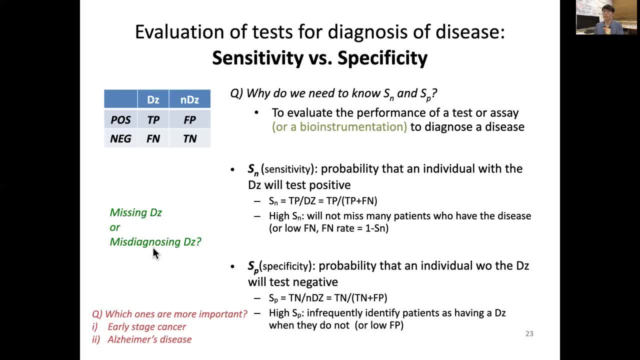 there's not much thing to do so in this. there's not much thing to do so in this case, case, case, in this type of disease, we don't want to, in this type of disease, we don't want to. in this type of disease, we don't want to misdiagnose. 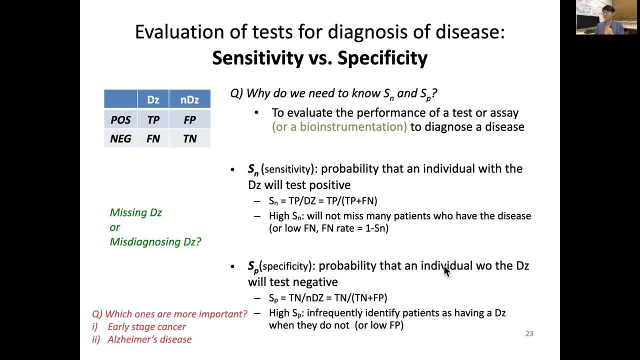 misdiagnose, misdiagnose. okay, so that i okay, so that i okay, so that i you know for i, for those patients who do you know for i, for those patients who do you know for i, for those patients who do not have disease, not have disease. 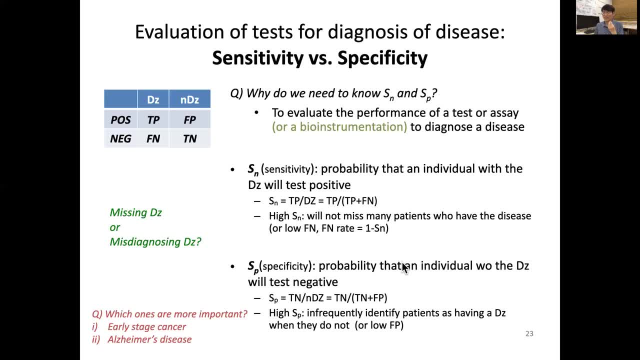 not have disease. don't want to get positive result in this. don't want to get positive result in this. don't want to get positive result in this case, case, case. what matters is high specificity. hopefully, what matters is high specificity. hopefully, what matters is high specificity. hopefully, this makes sense for you. 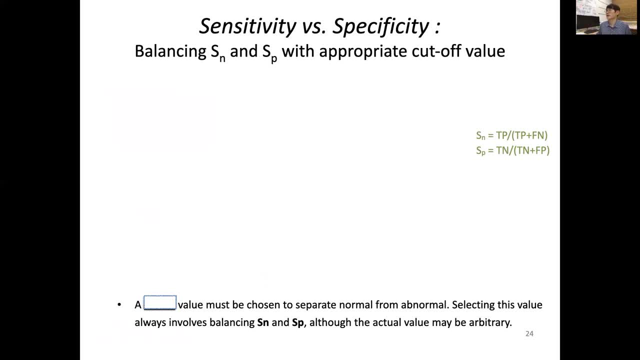 this makes sense for you. this makes sense for you. i want to get involved more about. i want to get involved more about. i want to get involved more about sensitivity and specificity. because sensitivity and specificity, because sensitivity and specificity, because when we, when we develop an instrument, when we, when we develop an instrument, 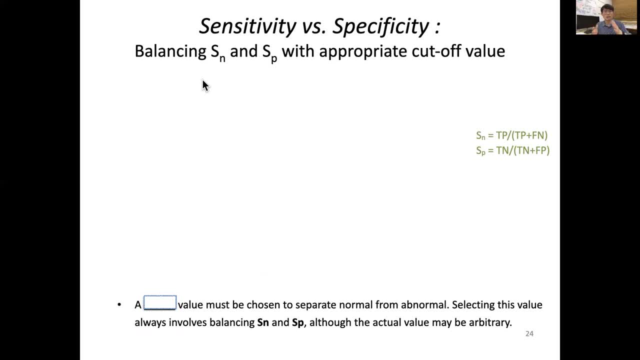 when we, when we develop an instrument, you somehow have to, you somehow have to, you somehow have to binarize or demarket, whether positive or binarize or demarket, whether positive or binarize or demarket, whether positive or negative, negative, negative, that threshold value is what you said. so 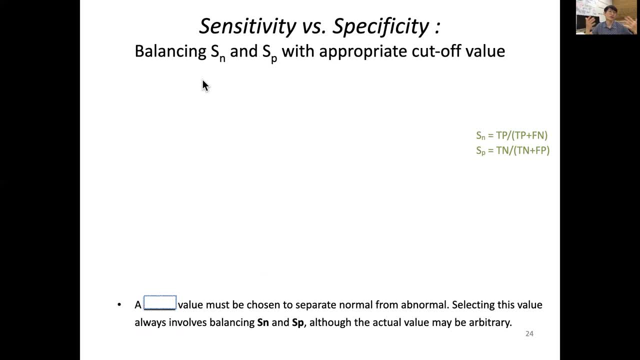 that threshold value is what you said. so that threshold value is what you said. so how to set the threshold, how to set the threshold, how to set the threshold. were it's an uh, it's important, so let's. were it's an uh, it's important, so let's. 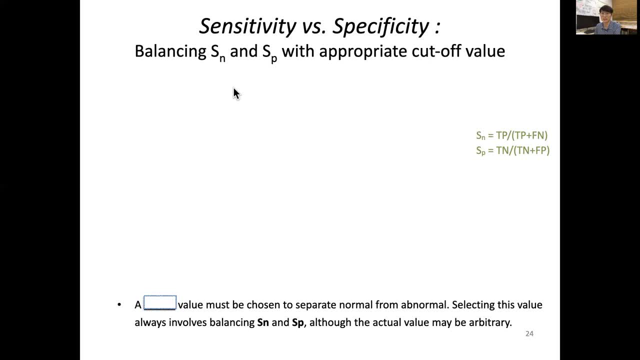 were, it's an uh, it's important. so let's see a practical case of a disease. and see a practical case of a disease. and see a practical case of a disease, and your instrument, your instrument, your instrument. so this x-axis is the test value of. so this x-axis is the test value of. 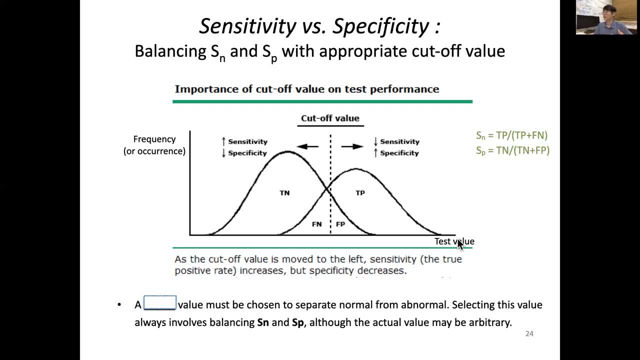 so this x-axis is the test value of quantitative value. your instrument will quantitative value. your instrument will quantitative value. your instrument will give out, give out, give out. okay. the y-axis is the frequency, the- okay. the y-axis is the frequency, the- okay. the y-axis is the frequency, the number of cases. 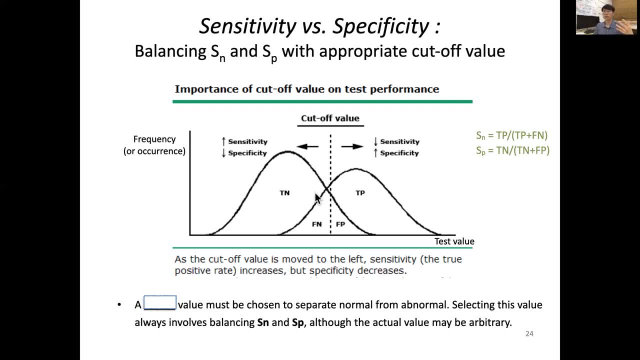 number of cases. number of cases. so then um in the, so then um in the, so then um in the true point of view in the disease there, true point of view in the disease there, true point of view in the disease, there will be, will be, will be. uh, you know, disease population. let's say: 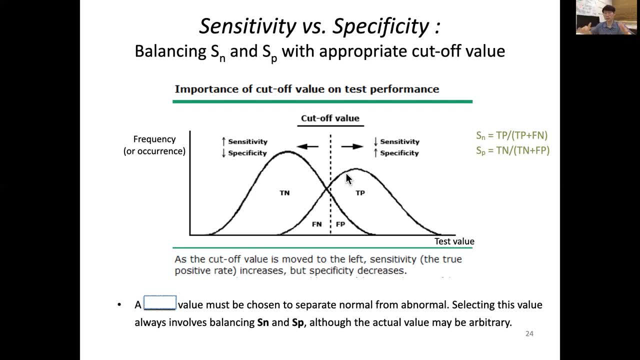 uh, you know disease population. let's say: uh, you know disease population. let's say: is- uh- in this case, it looks like a normal. is- uh, in this case, it looks like a normal. is- uh, in this case, it looks like a normal distribution, distribution, distribution which is having higher value. let's say: 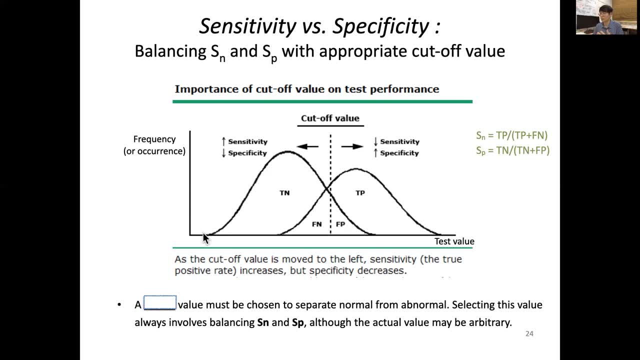 which is having higher value. let's say which is having higher value. let's say: and no disease will also have this and no disease will also have this and no disease will also have this population. but you notice that population, but you notice that population, but you notice that they are actually overlapping in general. 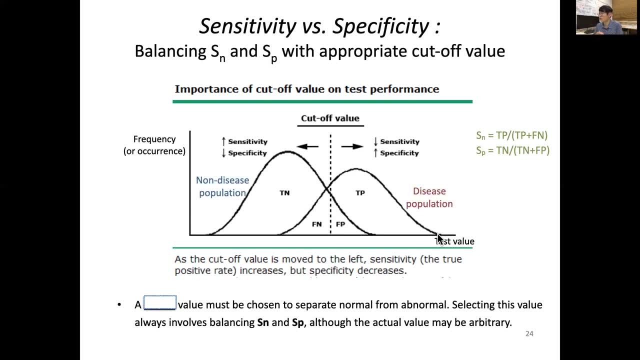 they are actually overlapping in general. they are actually overlapping in general. that is a the issue. so disease, that is a the issue. so disease, that is a the issue. so disease population: is this curve population? is this curve population? is this curve of distribution? non-disease population is. 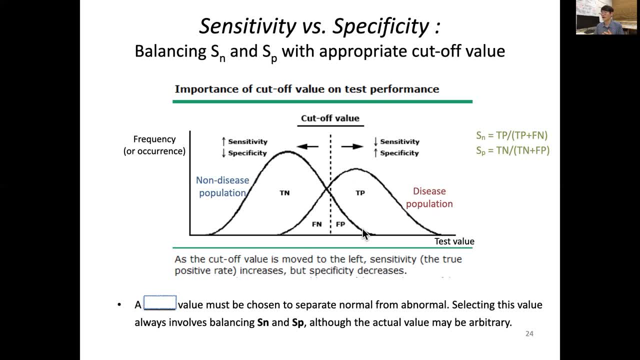 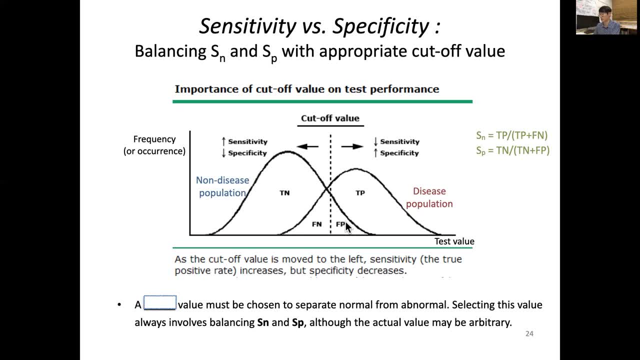 make a line, that one make a line, make a line that one bigger value of this line. you call it bigger value of this line. you call it bigger value of this line. you call it positive so that so positive, positive so that so positive, positive so that so positive and lower than this line. 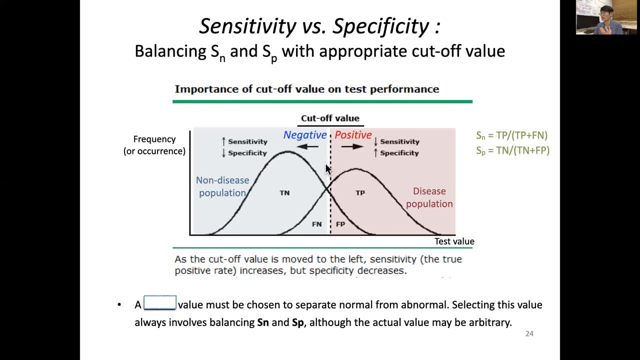 and lower than this line and lower than this line, your instrument will say hey, it's. your instrument will say hey, it's. your instrument will say hey, it's negative, negative, negative, and what you notice is positive, not only. and what you notice is positive not only, and what you notice is positive not only. have disease population. 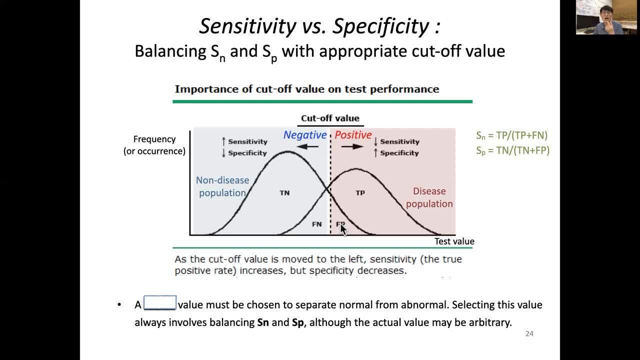 have disease population, have disease population, but also it's non-disease and this of, but also it's non-disease and this of, but also it's non-disease and this of course is called course, is called course, is called false positive, false positive, false positive for those non-disease population. 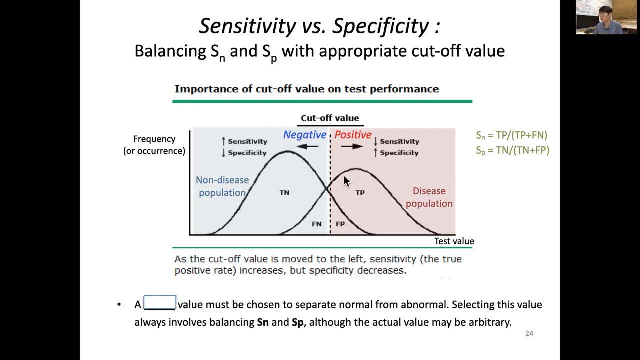 for those non-disease population, for those non-disease population, majority will be negative. but you see, majority will be negative. but you see majority will be negative. but you see, hey, even disease population can. hey, even disease population can. hey, even disease population can belong to negative. that means it is. 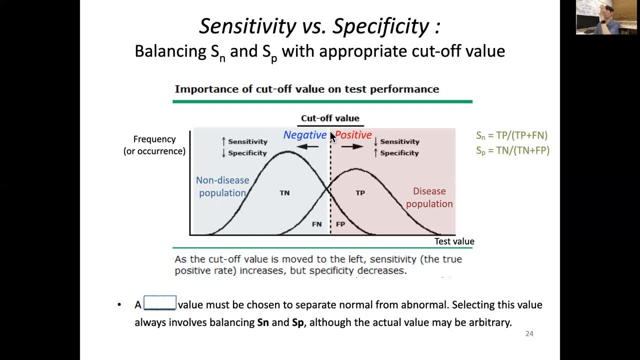 belong to negative, that means it is belong to negative. that means it is falsely negative, falsely negative, falsely negative. okay, so, okay, so, okay. so this value is called cutoff value, so this value is called cutoff value. so this value is called cutoff value, so that cutoff value must be chosen to. 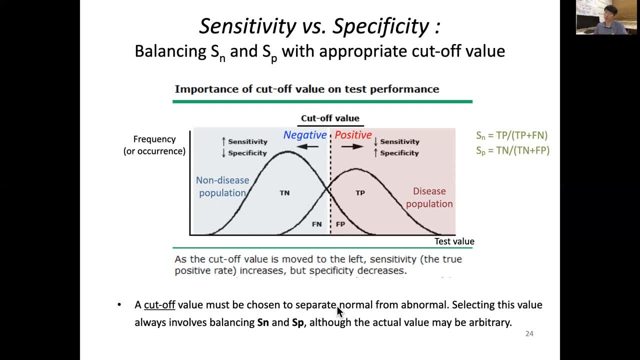 that cutoff value must be chosen to. that cutoff value must be chosen to separate normal from abnormal in this, separate normal from abnormal in this, separate normal from abnormal. in this case we call positive and negative case, we call positive and negative case, we call positive and negative. selecting this value always involves 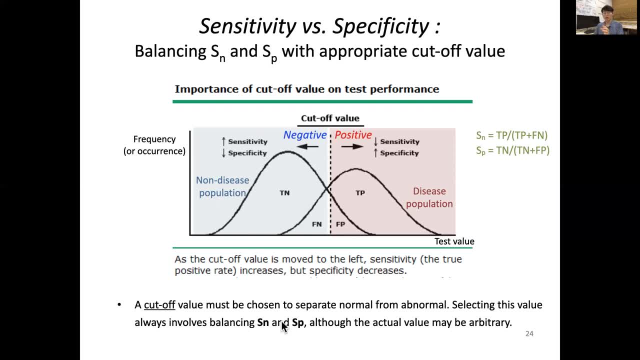 selecting this value always involves selecting this value, always involves balancing, balancing, balancing sensitivity and specificity, sensitivity and specificity, sensitivity and specificity, although the actual value may vary. so although the actual value may vary. so although the actual value may vary. so what does this mean? what does this mean? 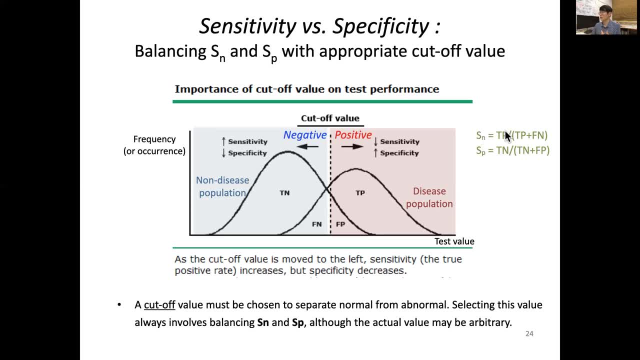 what does this mean? so we know from the definition of so, we know from the definition of so, we know from the definition of sensitivity, which is sensitivity, which is sensitivity which is out of disease, out of disease, out of disease, the portion of true positive, the portion of true positive. 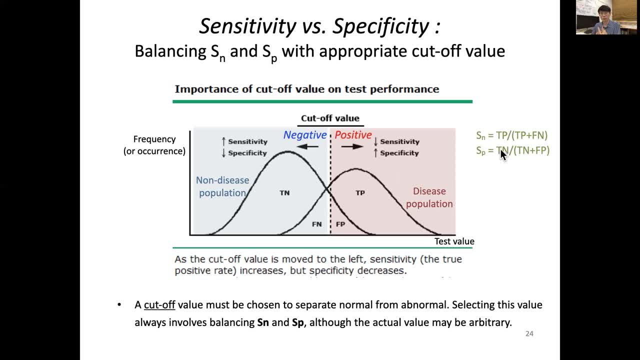 the portion of true positive specificity is out of non-disease, the specificity is out of non-disease, the specificity is out of non-disease, the proportion of true negative, proportion of true negative, proportion of true negative. so you can see here, let's say, if you 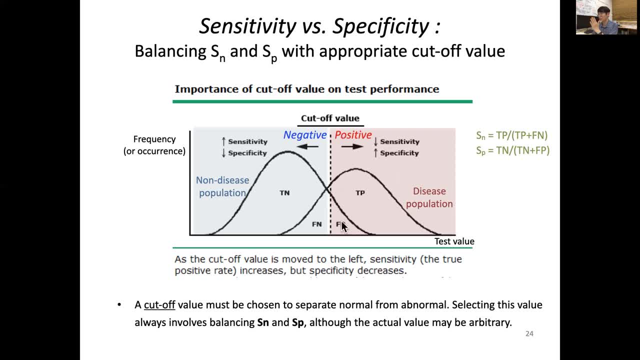 so you can see here. let's say: if you, so you can see here. let's say: if you have cutoff value, have cutoff value, have cutoff value to higher value, then you see false positive to higher value, then you see false positive to higher value, then you see false positive will be smaller. 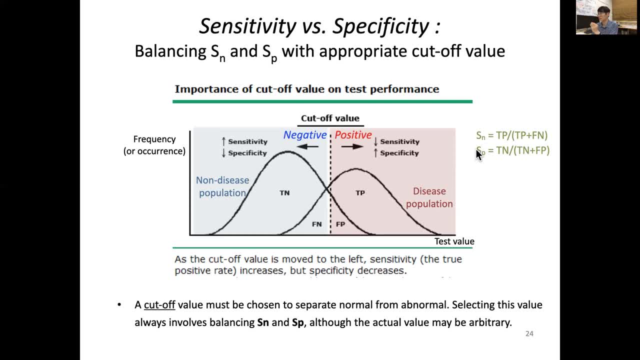 will be smaller, will be smaller and smaller false positive will increase and smaller false positive will increase and smaller false positive will increase. specificity, specificity, specificity: okay while okay, while okay, while false negative will increase, so that false negative will increase. so that false negative will increase. so that means sensitivity will decrease. 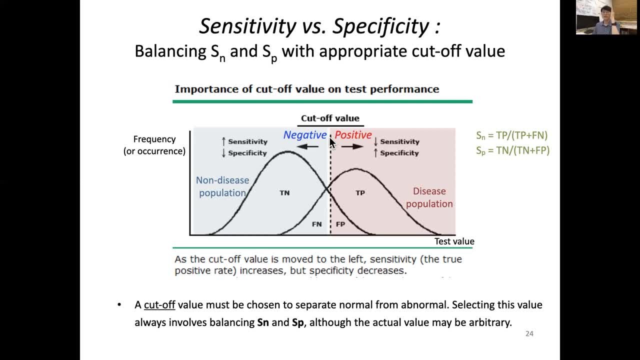 means sensitivity will decrease, means sensitivity will decrease. so you see the opposite effect of so you see the opposite effect of so you see the opposite effect of setting up your cutoff value higher. setting up your cutoff value higher. setting up your cutoff value higher will inevitably, will inevitably. 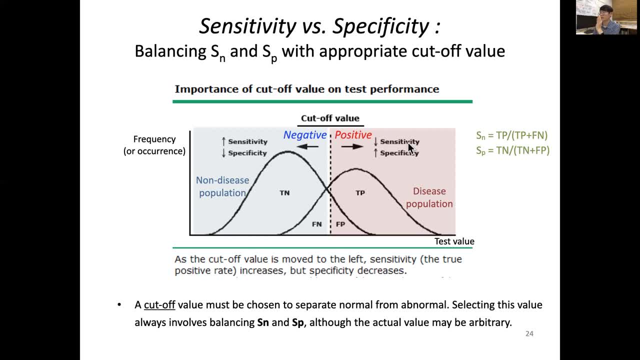 will inevitably needs higher specificity, while needs higher specificity, while needs higher specificity, while uh lowering sensitivity, uh lowering sensitivity, uh- lowering sensitivity, vice versa, if you put your cutoff value. vice versa, if you put your cutoff value vice versa, if you put your cutoff value lower, lower, lower than what happens will be, you can. 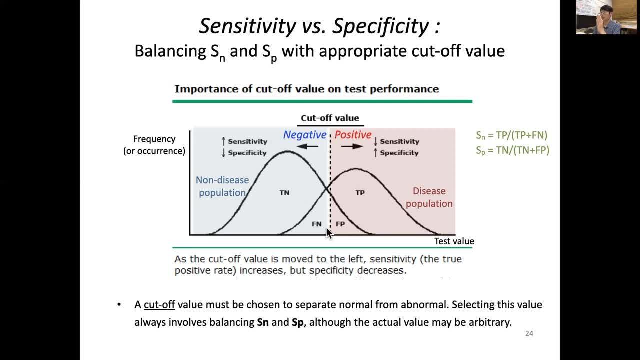 than what happens will be. you can, than what happens will be, you can increase, increase, increase sensitivity that you, you are really not sensitivity, that you, you are really not sensitivity that you, you are really not missing much disease, missing much disease, missing much disease, but your specificity will decrease does. 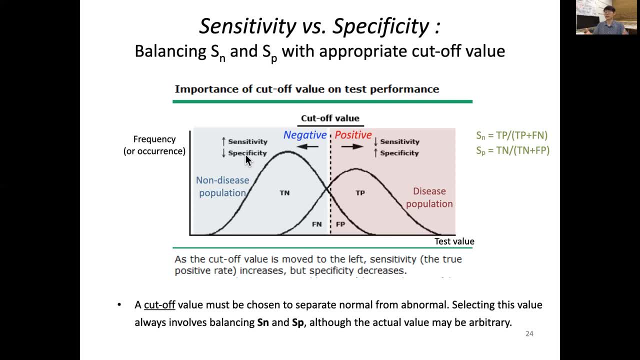 but your specificity will decrease. does, but your specificity will decrease. does it make sense? it make sense, it make sense. so it's like always, a compromise. there's, so, it's like always a compromise there's. so it's like always a compromise. there's nothing, nothing, nothing. you gain everything, right. 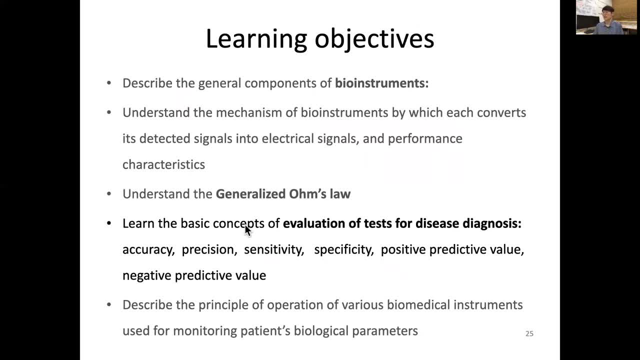 you gain everything right. you gain everything right. so, with this, so with this, so with this next time i'm going to discuss about more. next time i'm going to discuss about more. next time i'm going to discuss about more positive predictive value, positive predictive value, positive predictive value and negative predictive values. and negative predictive values and negative predictive values. thank you for your attention. thank you for your attention. 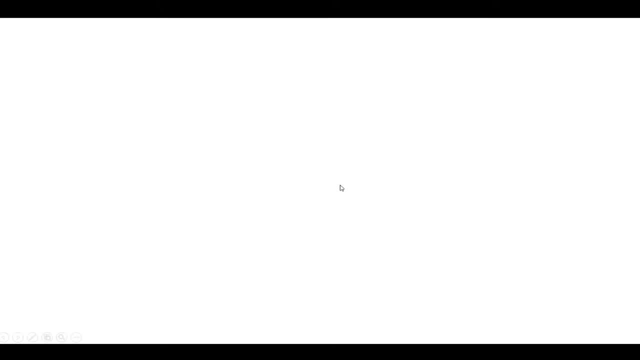 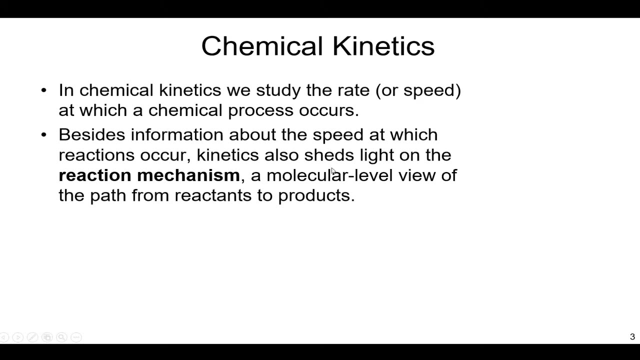 Okay, in today's lecture we're going to talk about kinetics And chemical. kinetics is the area of science where we study the rates at which a chemical process occurs. So this is usually what's associated with kinetics. People think of kinetics in chemistry. they think of the speed of